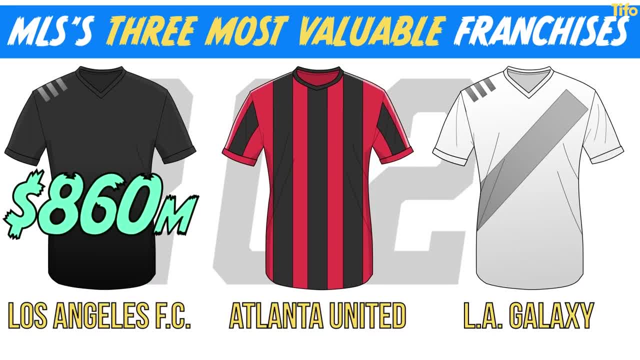 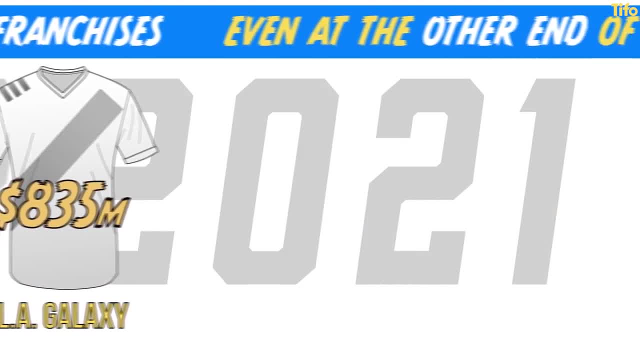 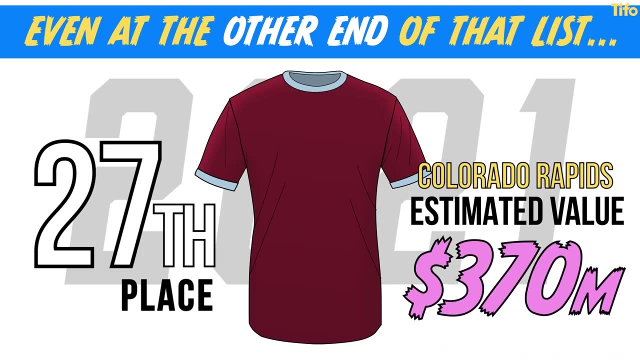 and LA Galaxy, valued at $860 million, $845 million and $835 million respectively. Even at the other end of the list, down in 27th place, the Colorado Rapids are estimated to be worth somewhere in the region of $370 million. In the overall context of North American sport, that's not much. 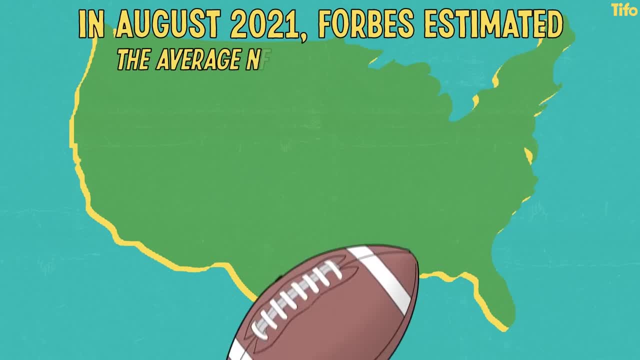 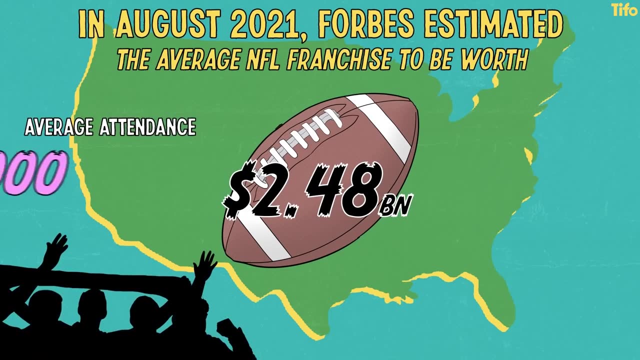 In August 2021, Forbes estimated the average NFL franchise to be worth $2.48 billion, But for a league in which the average attendance is just over 21,000, and the competition's broadcasting contract pays just $90 million per season, these are eyebrow. 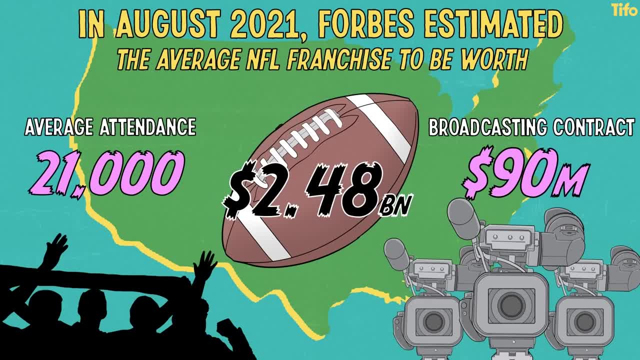 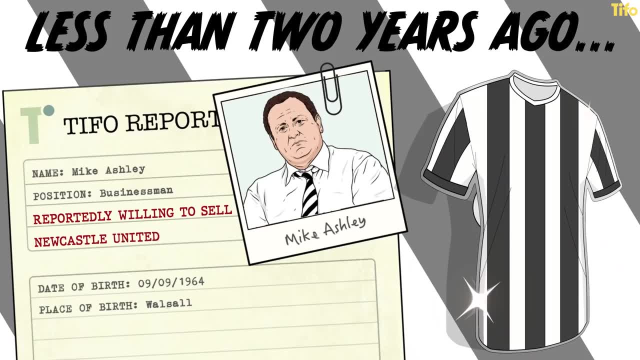 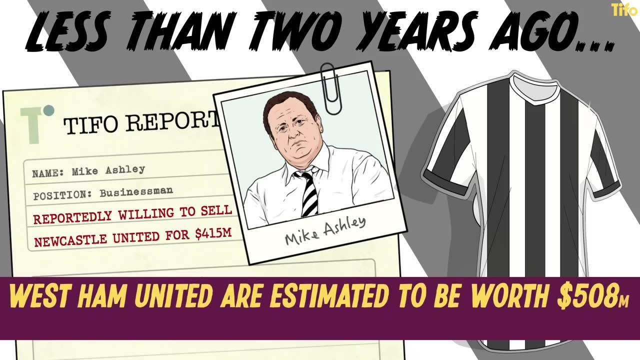 raising figures, particularly compared with other football. specific examples: Less than two years ago, Mike Ashley was reportedly willing to sell Newcastle United for $415 million, and West Ham United, who are currently subject to takeover interest, are estimated to be worth about $508 million, good enough for 17th place on Sportico's list. 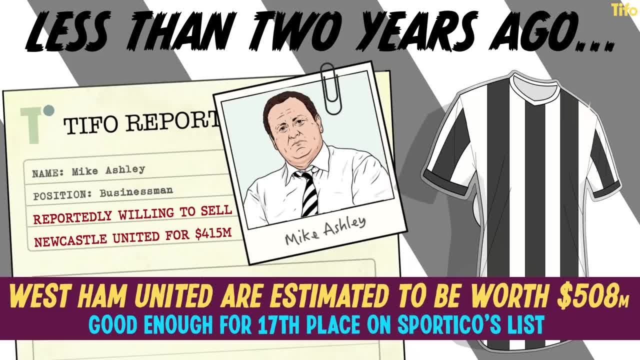 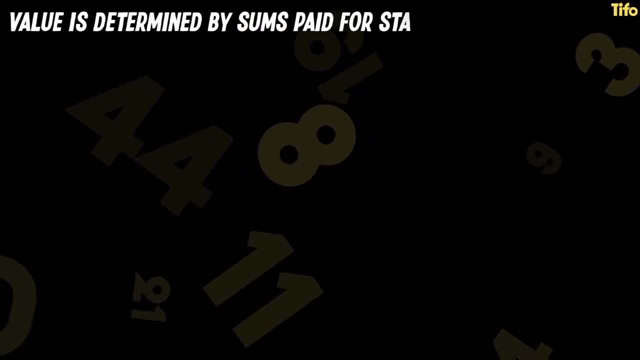 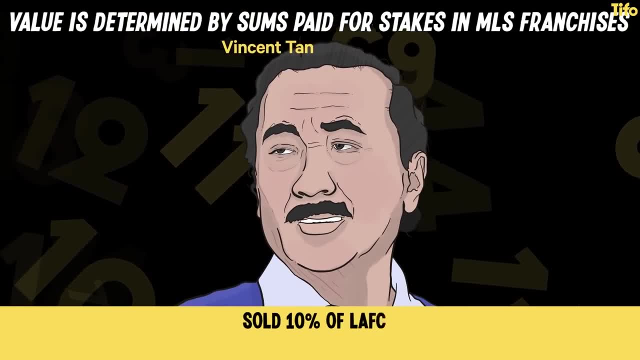 Can that be right And, if so, why and how? These numbers are just theory, of course, But such value is described by the actual sums paid for stakes in MLS franchises in recent years. In February 2020, Cardiff City owner Vincent Tan sold just 10% of LAFC for $70 million. 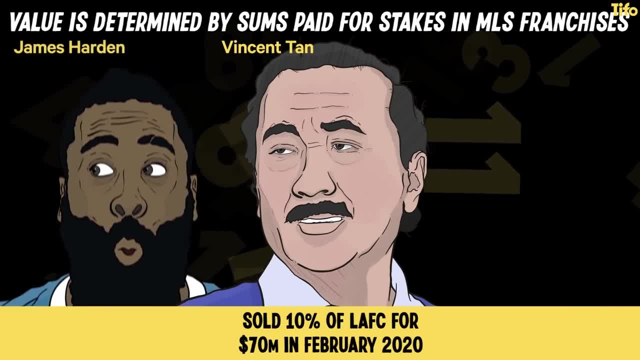 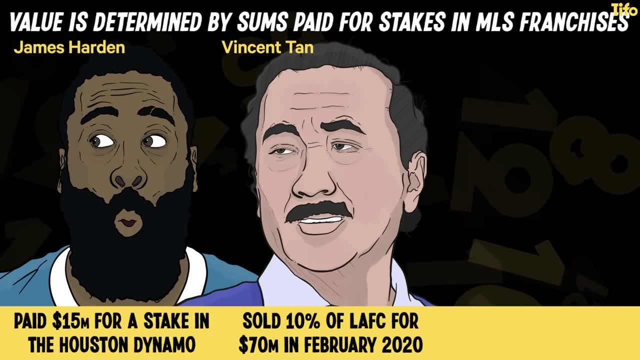 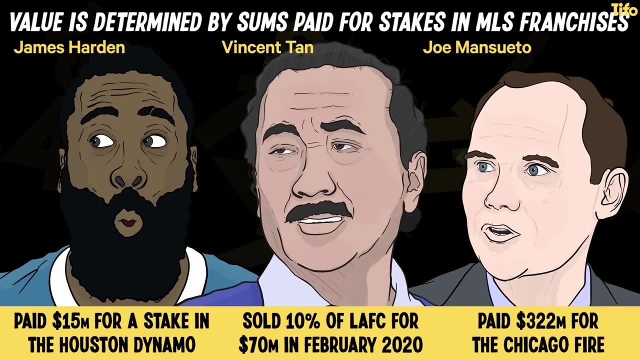 The previous year, in July 2019, NBA star James Harden purchased a minority stake in the Houston Dynamo for $15 million. A month before, in June 2019, Morningstar founder Joe Mansueto paid $322 million for ownership of the Chicago Fire. 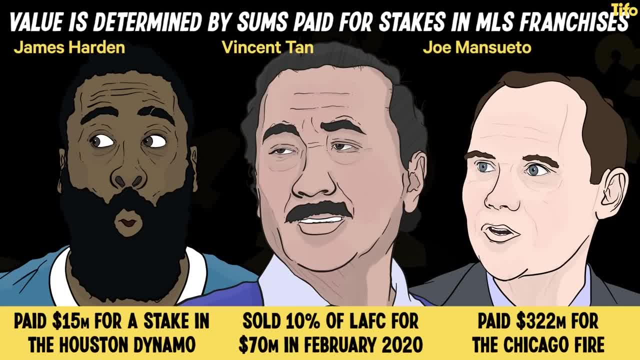 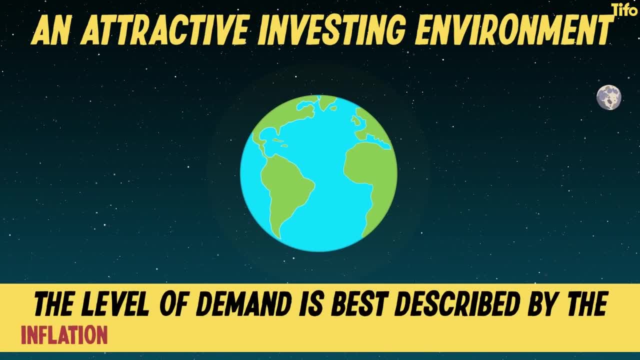 a team just three years removed from back-to-back wooden-spoon seasons. It's clearly an attractive investing environment and the level of demand is best described by the inflation in expansion fees MLS has been able to collect as the competition grows towards becoming a 29-team league in 2023.. Back in 2007,, Toronto joined MLS, having paid $10 million. The same yearsyunday's product Cardiff City also joined MLS. The same year, Syunday's product Cardiff City also joined MLS, having paid $10 million. The same year, Syunday's product Cardiff City also joined MLS. The same year, Syunday's product Cardiff City also joined MLS. 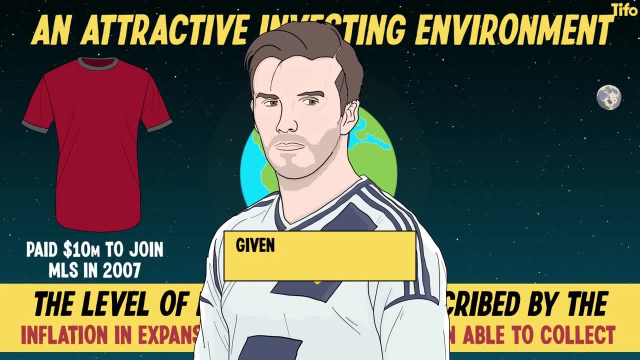 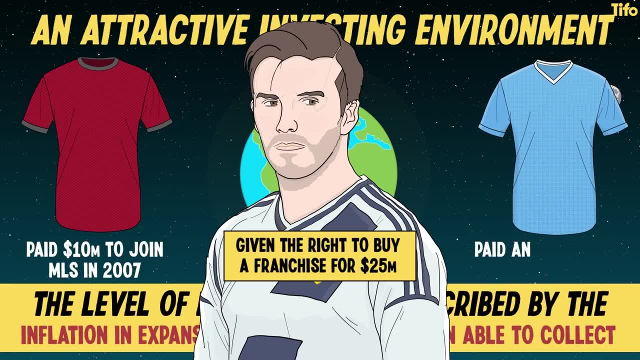 The same year, Syunday's product, Cardiff City, also joined MLS. Same year, as part of his playing contract, David Beckham was assured the right to purchase a future franchise for $25 million. These were quaint fees In 2013,. New York City FC. 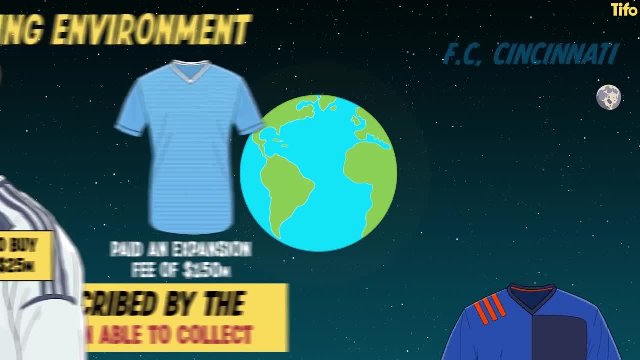 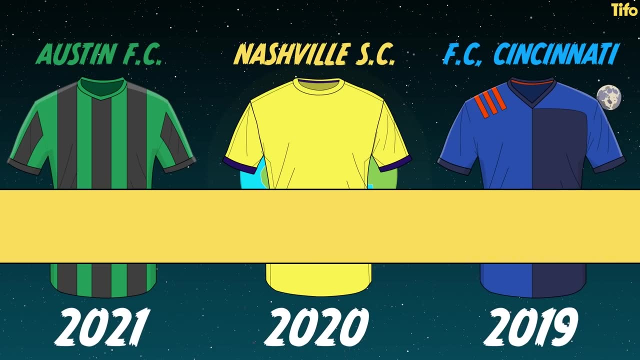 paid an expansion fee of $150 million, as did Cincinnati in 2019, Nashville in 2020 and Austin in 2021.. In 2022, Charlotte FC will take their place in the league, and it will be after David Tepper. 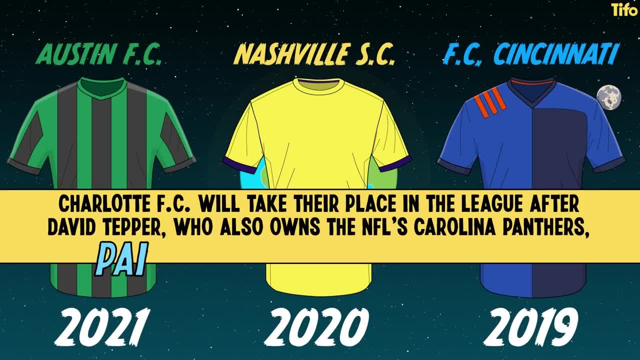 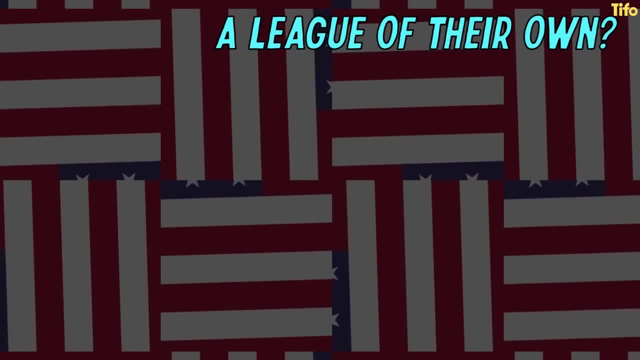 who also owns the NFL's Carolina Panthers, paid a staggering $325 million. It's a trend that makes MLS an outlier even in the hyper-capitalist world of US sport. According to a March 2021 article written by the Athletics' Sam Stedgill, the average 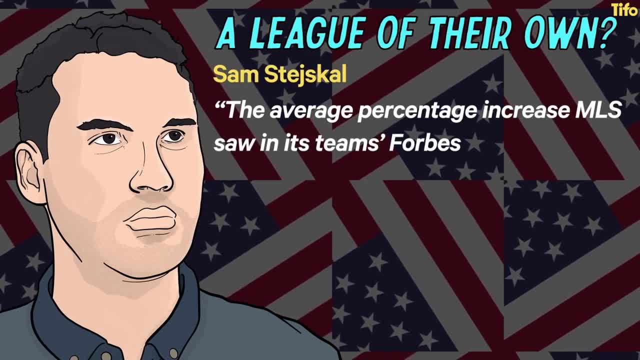 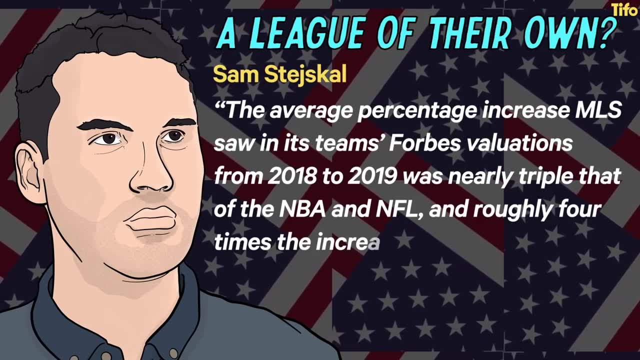 percentage increase MLS saw in its team's Forbes valuations from 2018 to 2019 was nearly triple that of the NBA and NFL And roughly four times the increases seen in MLB and NHL, including the NBA and NFL, in the same period. 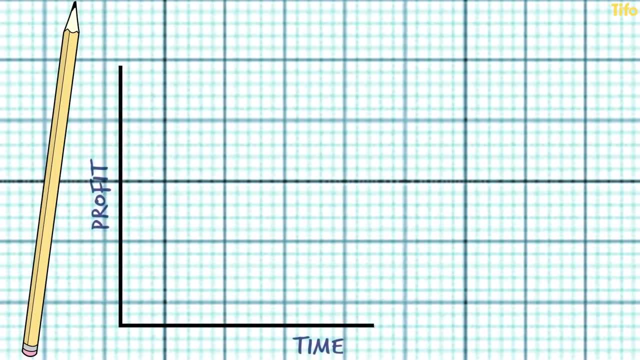 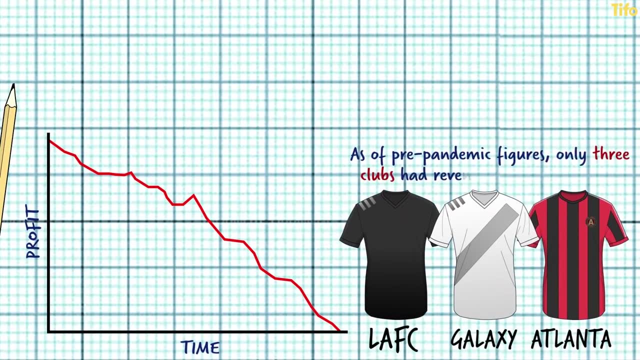 It's an amazing figure, especially so given that very few of the franchises are profitable and that, as of pre-pandemic figures, only three clubs had revenues in excess of $50 million. In fact, in 2018, the 23 teams that took part made a collective loss of $100 million. 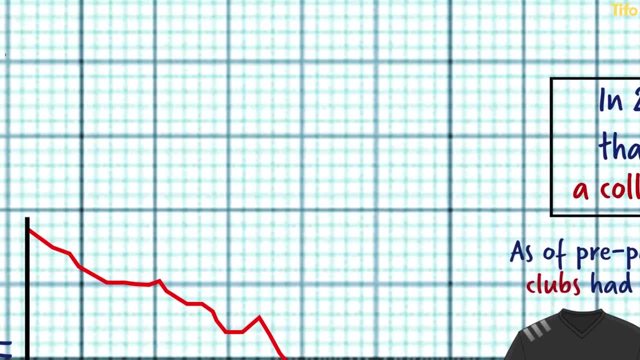 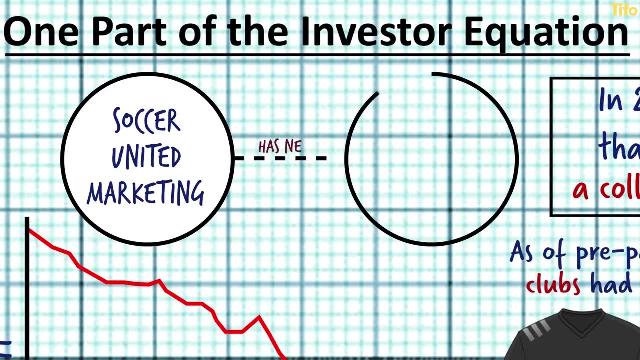 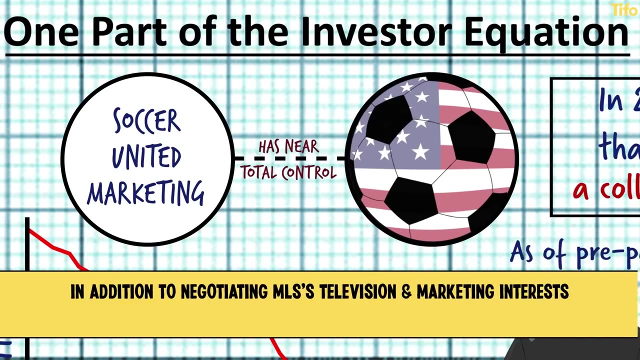 But the revenues earned by the individual franchises are only one part of the investor equation. With ownership comes stakes in Soccer United Marketing. a subsidiary of the United Basketball Association, It has near total control over soccer's commercial interests in the United States. In addition to negotiating MLS's television and marketing interests, it also handles the 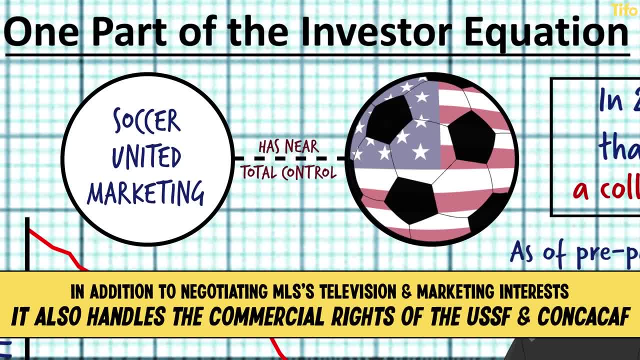 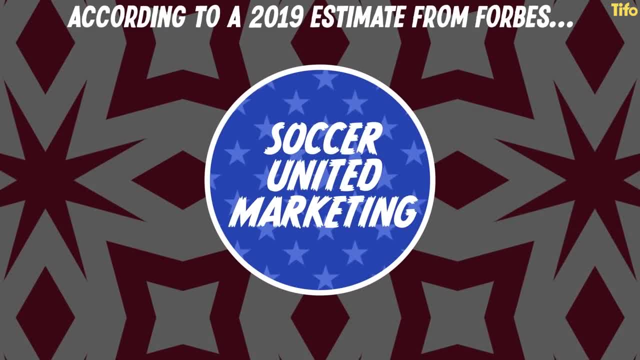 commercial rights of the USSF and CONCACAF, And it's lucrative. According to a 2019 estimate from Forbes, SUM, which is wholly owned by the league investors, is worth around $2 billion, with annual revenues of $350 million. 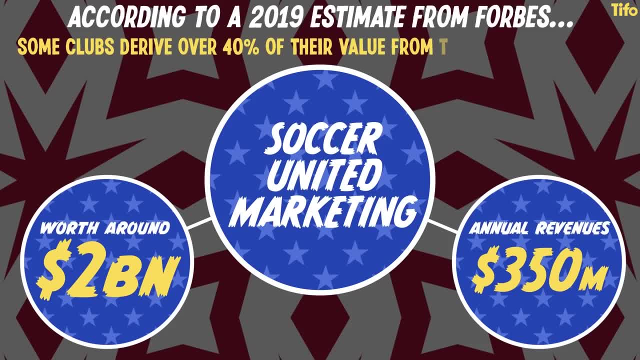 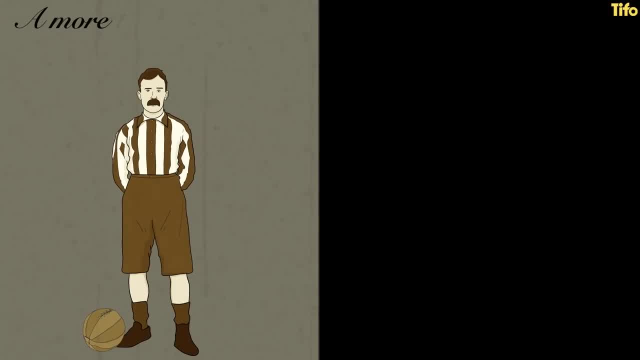 And it's estimated that some clubs derive more than 40 per cent of their value from those holdings alone. It creates a distinction between the variety of ownership found in European football, which is a more traditional kind of stake-holding tied to a team's rise and fall, and ownership 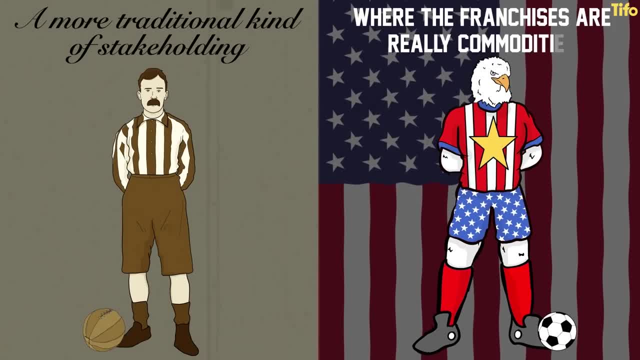 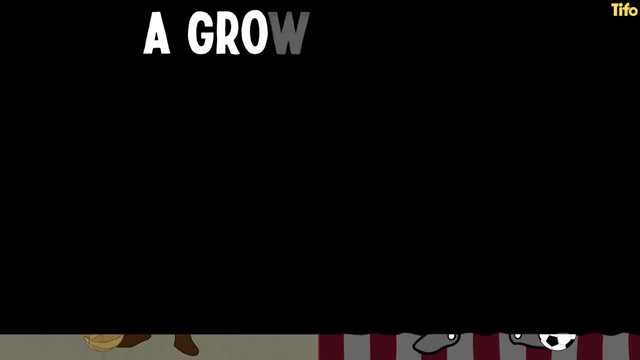 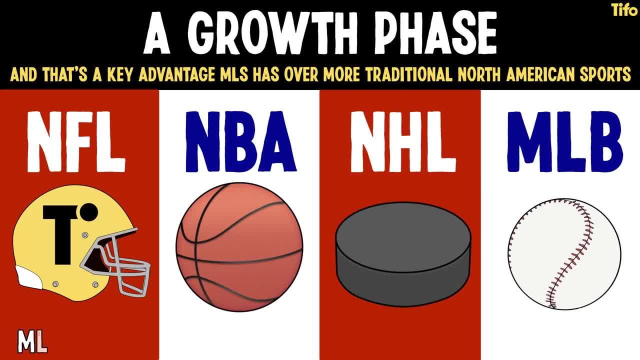 sport. The MLS is a more traditional, more competitive sport. The MLS is a more traditional sport. The MLS is a more traditional, more competitive sport. Rather than twist breaking, MLS, Att, Delta and MLB soccer is nowhere near reaching its potential, yet there's every reason to believe it will continue to push towards it – and for reasons. 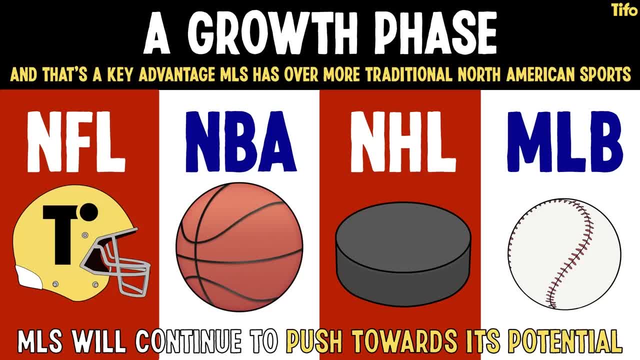 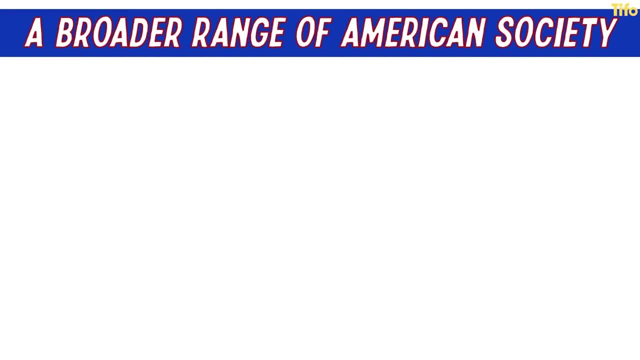 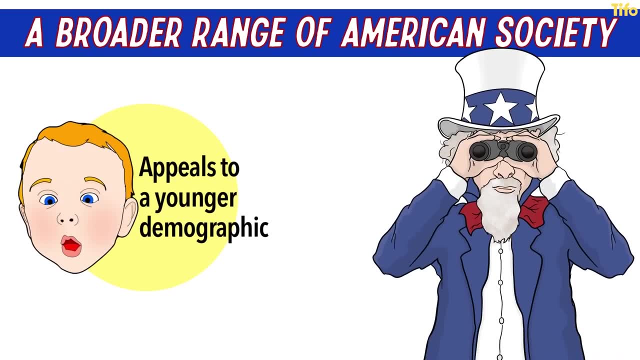 beyond just the big boisterous crowds in Atlanta and Seattle. Soccer theoretically appeals to a broader range of America's society and to its vast Hispanic population, But it's also favoured by a younger demographic too. A 2019 survey carried out among US watchers of the English Premier League discovered that 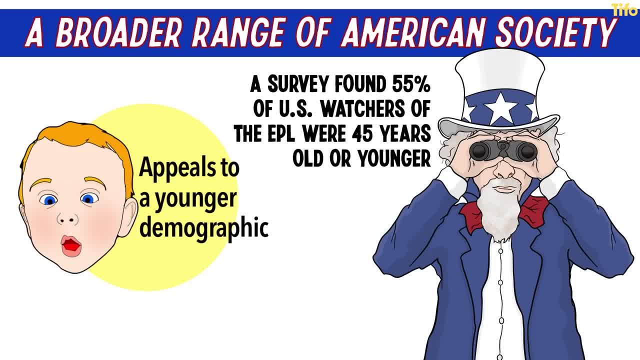 over 55 per cent were 45 years old or younger. 6.oken and Loris Rudd, second boy, are rather more 55 per cent older than position numbers of MLS. 5.Checketing results: Last season broadcaster NBC reported an average total viewership across their various platforms: 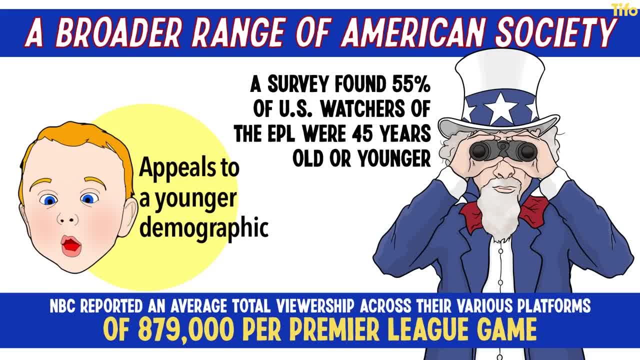 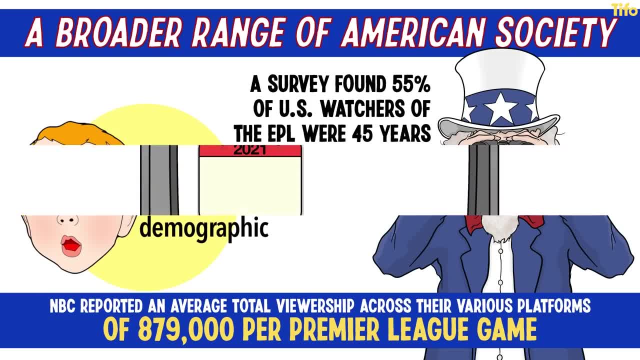 of 879,000 per Premier League game, which was both a 2% rise on the year before and double that of the average NHL broadcast In July 2021,. 9.4 million viewers also watched the European Championship final between England. 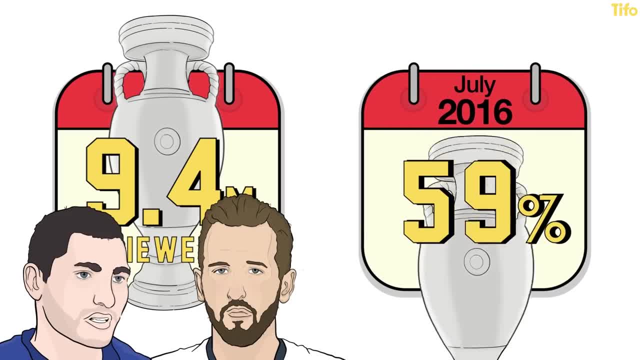 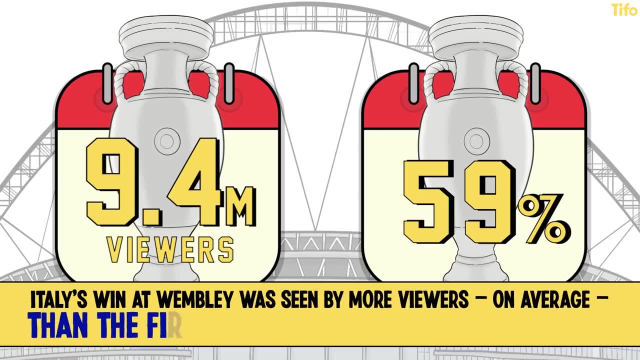 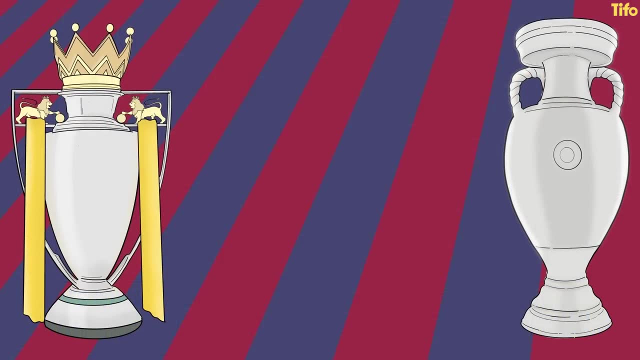 and Italy, a 59% rise on the 2016 final between Portugal and France. Italy's win at Wembley was also seen by more viewers than, on average, watched the first three games of the NBA Finals. Of course, the Premier League and European Championship are not MLS, but their audiences. 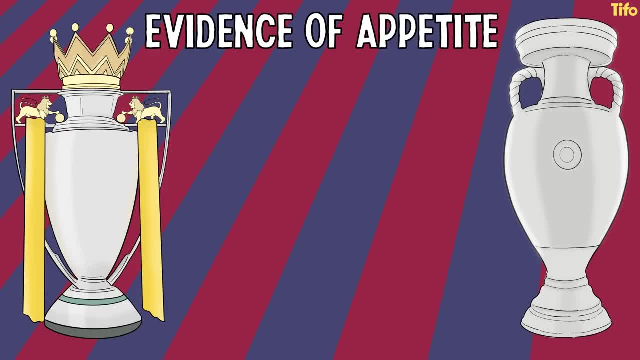 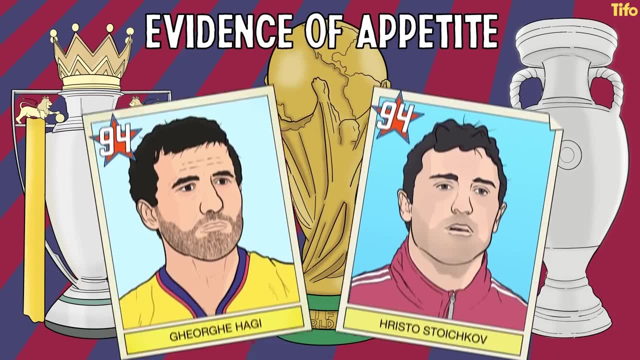 provide evidence of appetite, and the US isn't far away from hosting its second World Cup alongside Canada and Mexico in 2026.. In 1994, the momentum generated led to MLS's original launch, and the expectation this time is for a much bigger jolt. 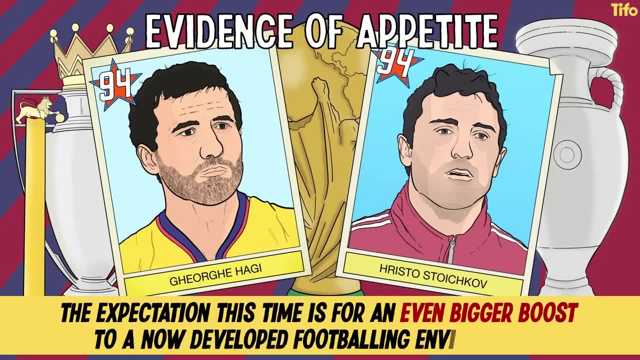 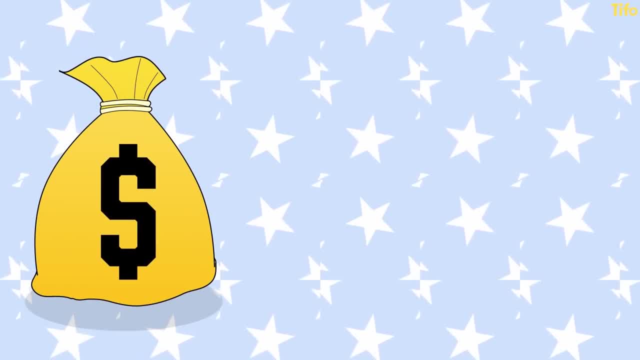 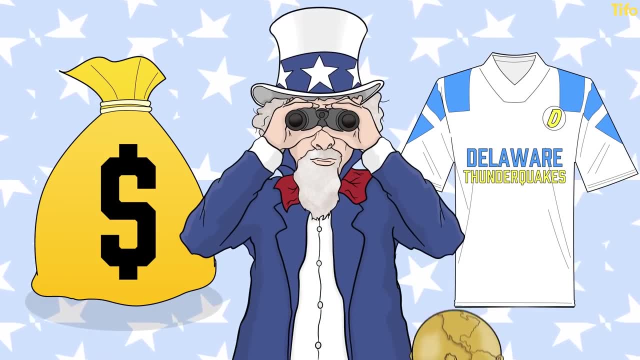 And presumably an even bigger boost to a now-developed footballing environment. They are caveats, of course. Expansion, and the revenues associated with it, cannot carry on forever, not without damaging the quality of the league And, more importantly, while US eyes will doubtless be drawn to the World Cup, MLS franchises.